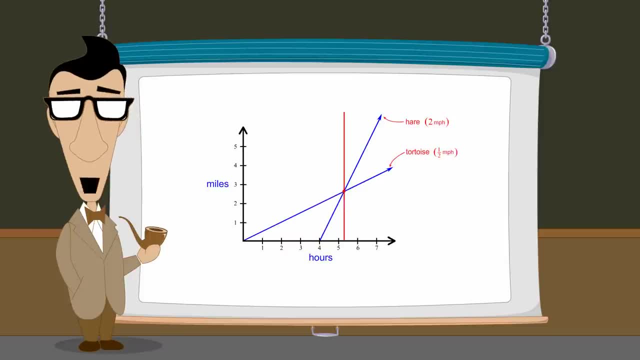 once he started, he quickly caught up, eventually passing the tortoise some time between five and six hours after the race had begun. At the end of the lecture, we derived equations for these graphs. In this lecture, we will see how to use these equations. 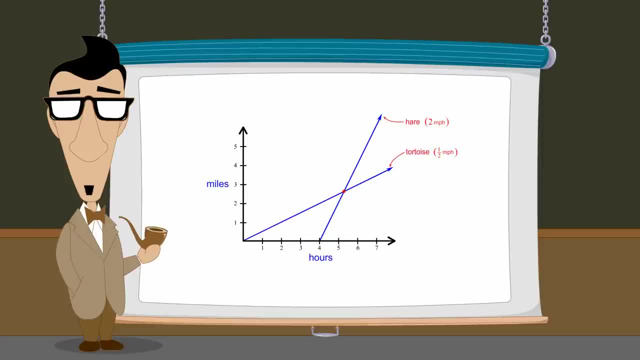 to mathematically determine the coordinates of their intersection point and thus the exact time and distance when the tortoise and hare meet. There are several different mathematical methods which can be used to find the points of intersection of two graphs. In this lecture, we will demonstrate a method. 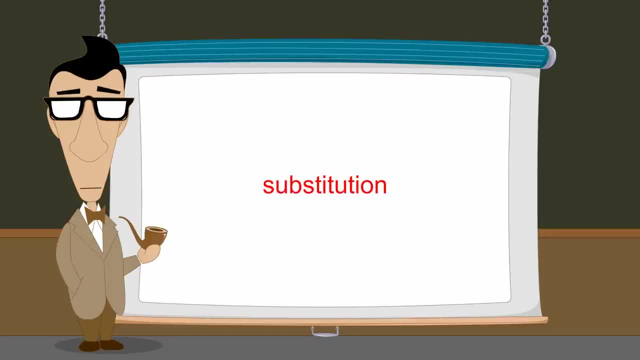 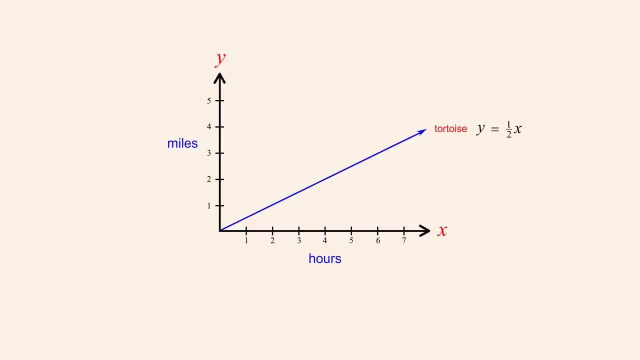 In this lecture we will demonstrate a method called substitution. We know that the coordinates of any point on an equation's graph represent one possible solution to the equation. So the set of all points which make up the graph represents every possible solution to the equation. 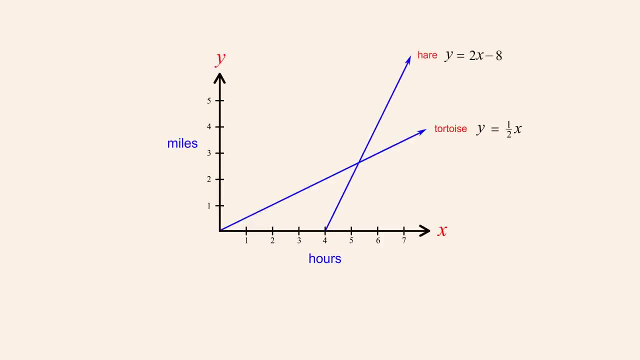 Likewise for a different equation, the set of all the points which make up that graph represents every possible solution to that equation. Any point which lies on both graphs therefore represents a solution to both equations. We can find this intersection point if we find values for x and y. 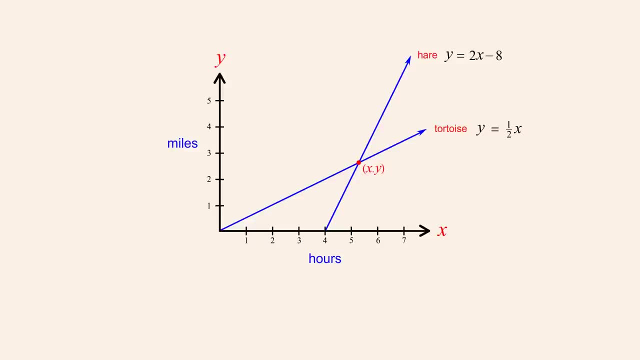 which simultaneously satisfy both equations. Each equation tells us something about the relationship between x and y. For example, the second equation tells us that the value of y must be equal to one half of x. For example, the second equation tells us that the value of y must be equal to one half of x. 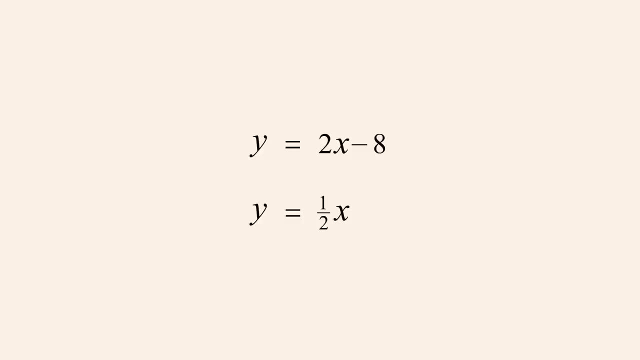 Since we know that the value of y must be one half x, we can substitute one half x for y in the first equation. This gives us an equation with a single variable, x. We can then solve this equation to find the value of x Multiplying both sides by two. 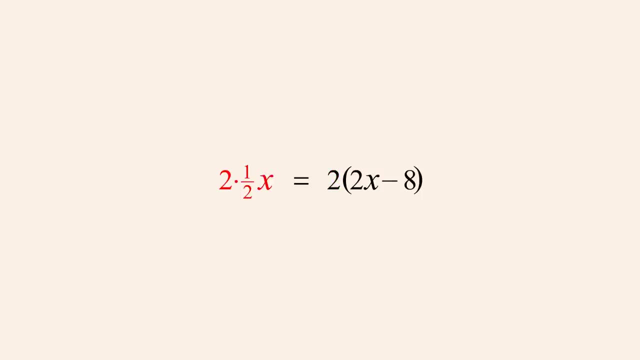 on the left we get two times one half x or x, and on the right, distributing the two to the terms in parentheses, we get two times two x or four x minus two times eight or sixteen. Adding sixteen to both sides and subtracting x from both sides. 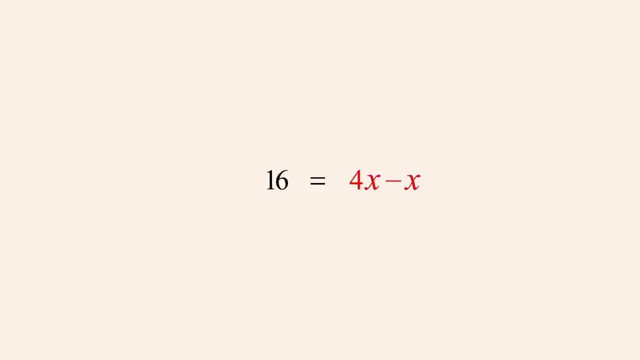 we get sixteen equals four x minus x, or sixteen equals three x. Finally, dividing both sides by three gives us sixteen thirds equals x or x equals sixteen thirds. Now that we know the value of x, we can set the value of x in either equation to sixteen thirds. 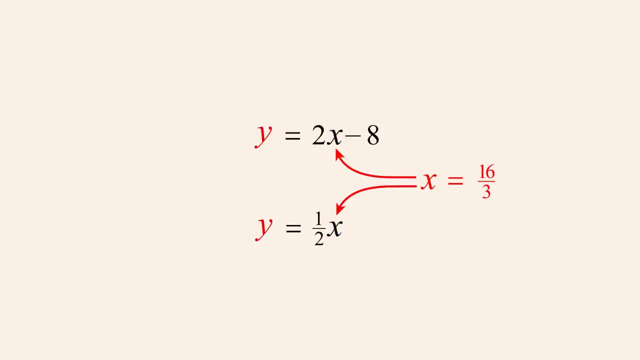 and find the corresponding value of y. Either equation will give us the same answer. so since the second equation is the simplest, we will use it to find the value of y. Setting x to sixteen thirds, we see that y is one half times sixteen thirds, or eight thirds. 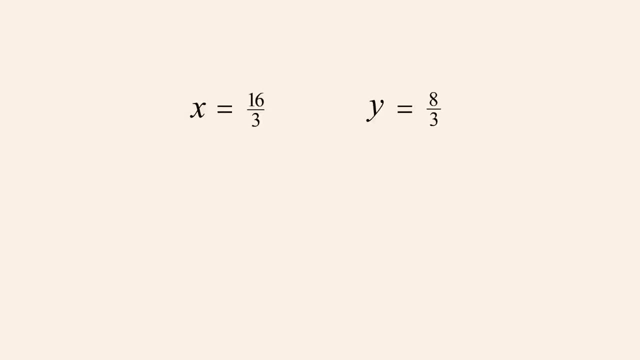 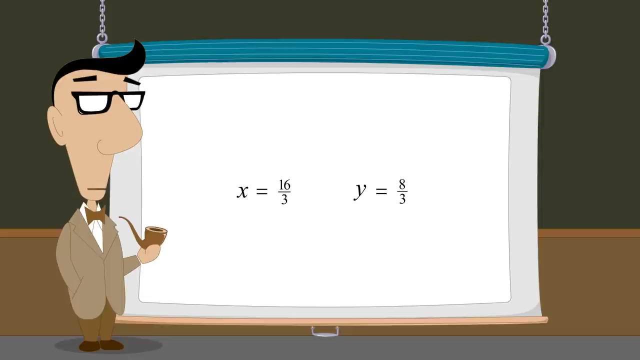 We can check our calculated values for x and y by substituting them for x and y in the original equations and verifying that they create true statements. So the values of x and y which satisfy both equations are sixteen thirds and eight thirds. These are the values of the x and y coordinates. 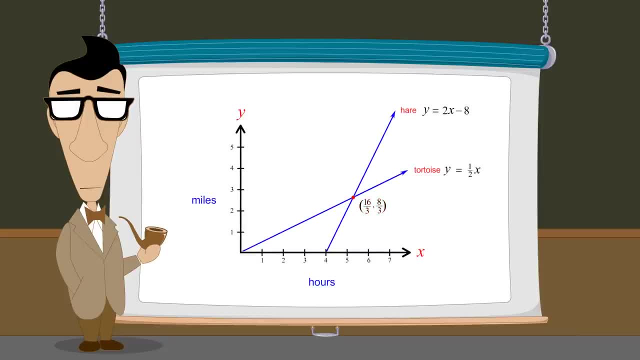 of the intersection point of the two graphs. Converting these fractions to mixed numbers, we see that this point represents an elapsed time of five and one third hours and a distance of two and two thirds miles from the starting point, So five hours and twenty minutes after the race has begun. 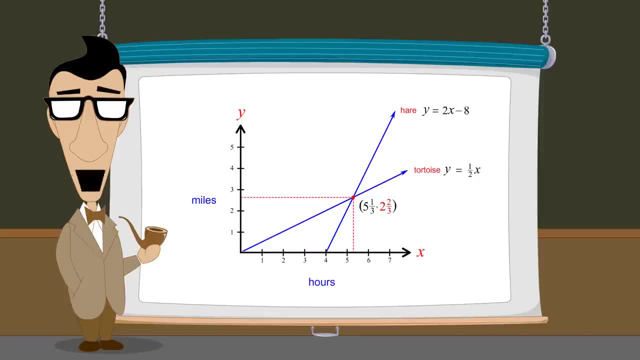 the tortoise and hare meet two and two thirds miles from the starting point. This method of solving a system of equations is called substitution. This name is appropriate since, as we saw in this example, the value of y represented in terms of x in one equation.